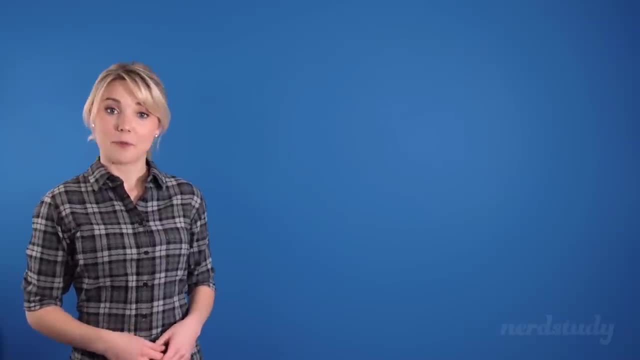 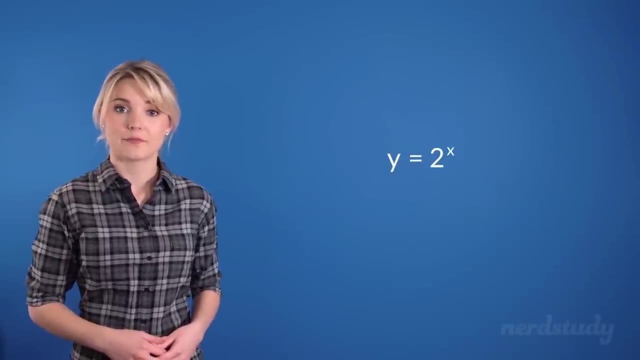 In an exponential function, however, the x-value is the exponent itself. An example of an exponential function would be: y equals 2 to the exponent x. As you can see, If x is 0, y is 1.. If x is 1, y is 2.. 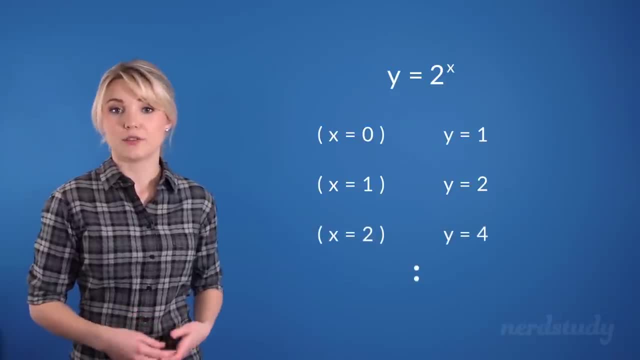 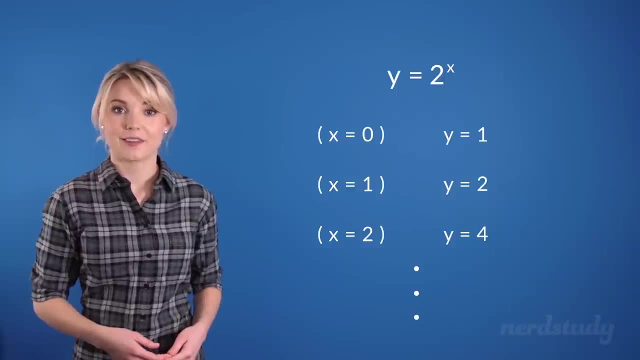 If x is 2,, y is 4, and so on and so forth. Notice how, as x increases, the increase in y itself becomes greater and greater. This is one of the key things about exponential functions, in that the graph increases at an increasing rate. 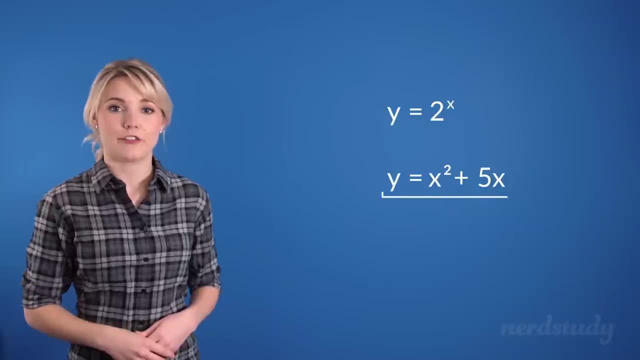 It's important to look at the equation of a quadratic function and look at the difference between that and our example of an exponential function. So let's look at the equation of a quadratic function and look at the difference between that and our example of an exponential function. 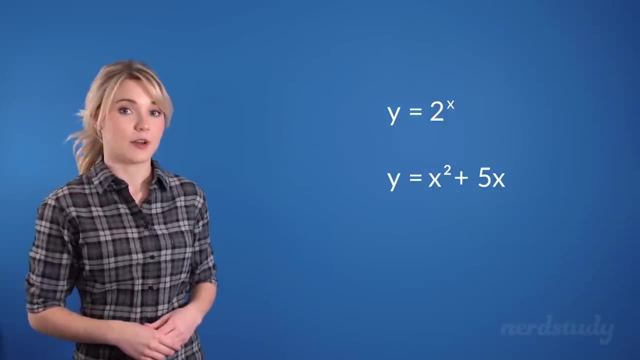 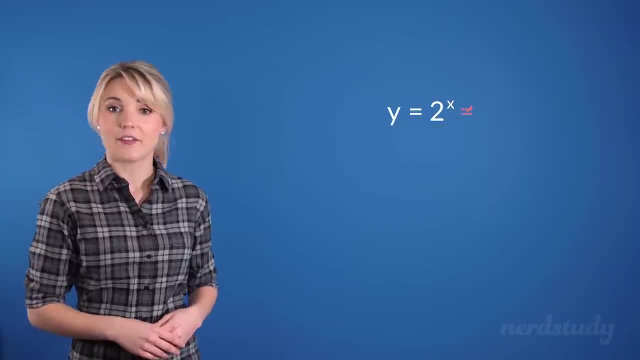 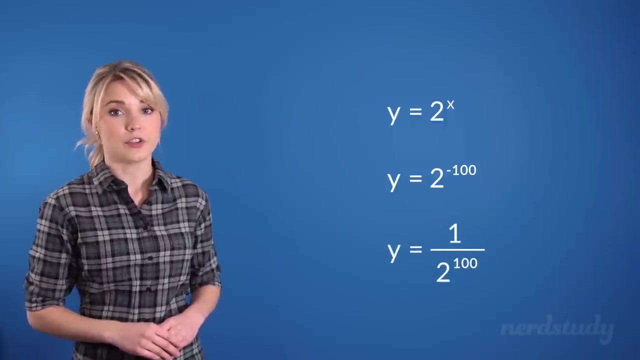 Notice how this quadratic function can equal 0 simply by making x equal to 0 in this example, However, our exponential function can never equal 0. Even if we did 2 to the exponent of negative 100, we would end up with 1 over 2 to the exponent 100,. 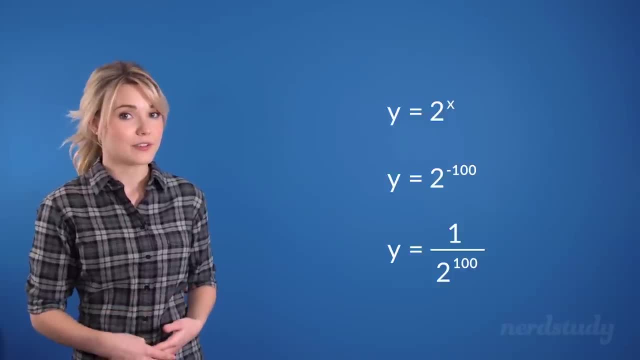 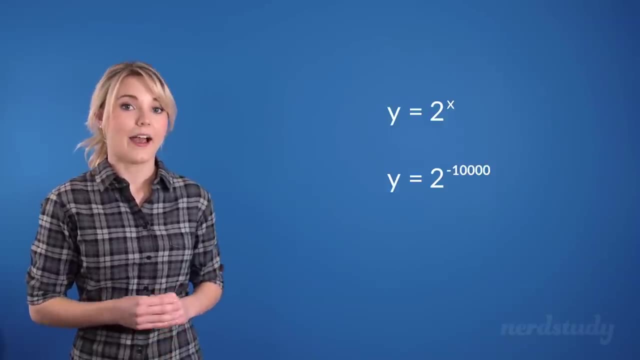 which is a very, very small number, getting very close to 0, but still never actually touching 0, since, once again, no matter how small we make the exponent, a negative exponent will simply result in a fraction, with the numerator equaling to 1.. 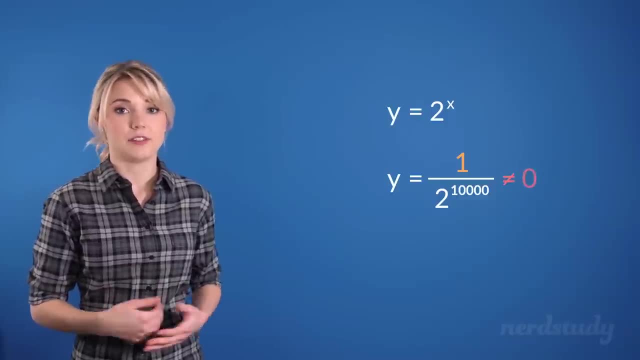 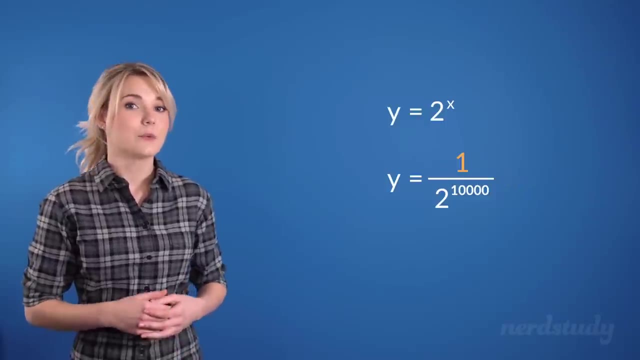 And this, right off the bat, means that it will not ever equal to 0.. We know this because a fraction only equals 0 when the numerator is a 0.. Good, So we can already see differences between the two functions, and it's important that we don't confuse the two. 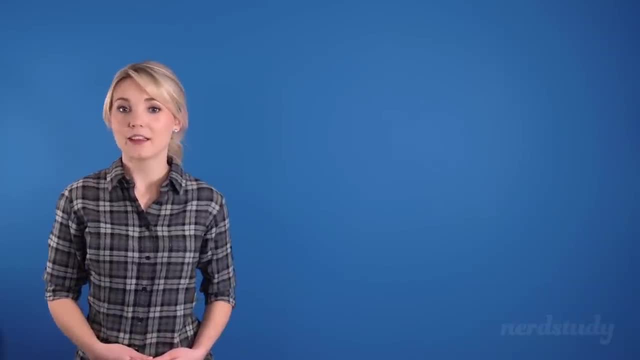 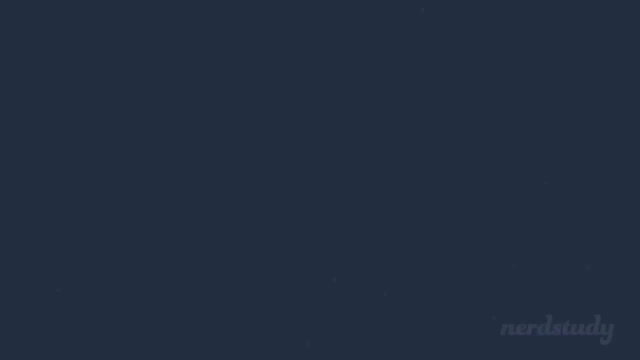 Now, before we finish off this video, let's quickly explore a bit more about exponential functions and what they actually look like. Here's an example of a generic exponential function. Now, if a is greater than 0 and b was greater than 1, then we can expect the graph to look something like this: 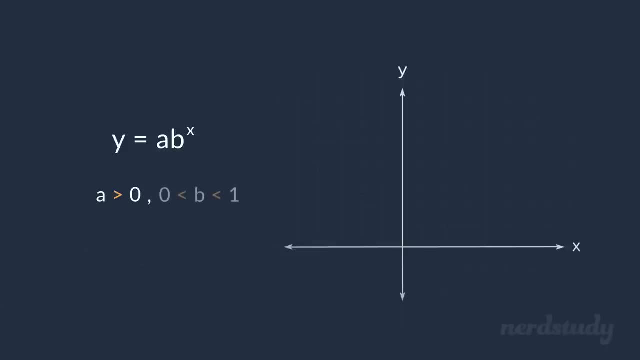 If a is greater than 0 and b is greater than 0, but less than 1,, then the graph will look something like this: Now, if a is less than 1,, then the graph will look something like this: If a is less than 0 and b was greater than 1,, then we can expect the graph to look something like this: